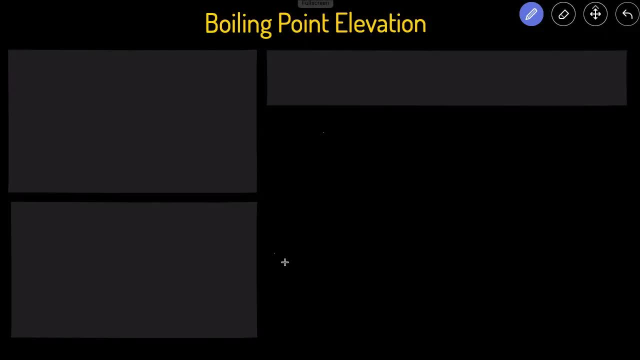 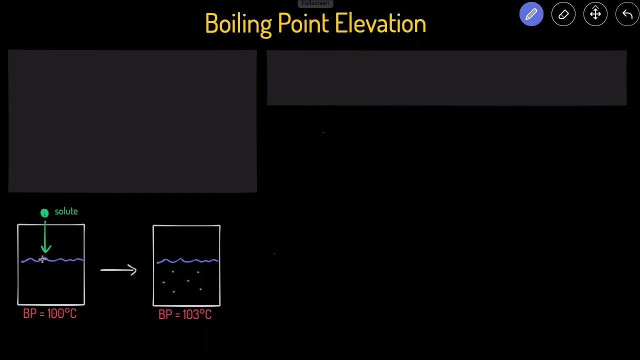 Hey guys, Michael from Kakao Chemistry, In this video we'll be going over boiling point elevation, what it is, what equations associated with it and several problems about how to use the equation. First of all, boiling point elevation. the concept is: if you have a solvent- in this case, let's pretend we have water which has a boiling point of 100 degrees Celsius and then we add some solid to it. that's going to create a new solution with a boiling point that's higher than the original boiling point. 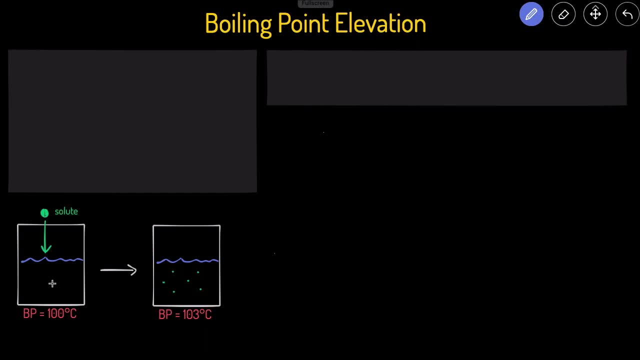 So, essentially, by adding a solute into the solvent, you're elevating the boiling point, and just the more solute that you add, the higher the boiling point of the final solution will be compared to the original solvent. The equation that you use for boiling point elevation is written here: 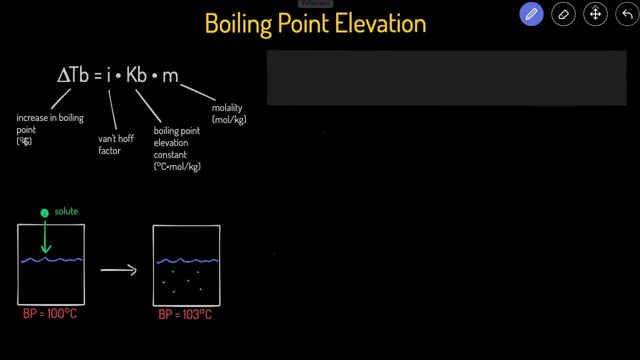 Change in the temperature of the boiling point, which is typically in degrees Celsius, is equal to I, which is the Van Gogh factor, which is how many species the solute will break up into. Don't worry, this will make it a little bit more clear. 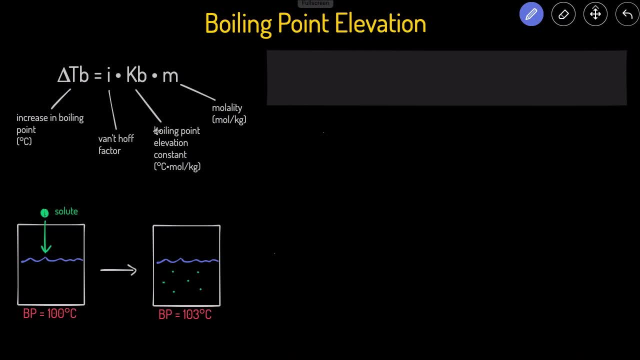 When we look at the example problem, multiply it by Kb, which is the boiling point elevation constant, which is going to be different for every solvent, and multiply it by the molality lowercase, m, which is equal to the moles of the solute divided by the kilograms of the solvent. 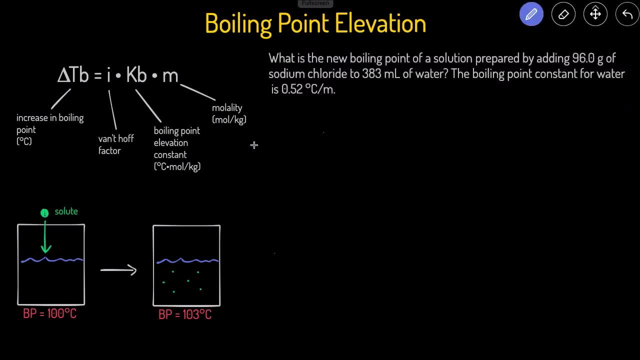 All right, let's take a look at how we can use this equation in the problem. So this problem is asking us what is the new boiling point of solution that's prepared by dissolving 96 grams of sodium chloride to 383 milliliters of water. 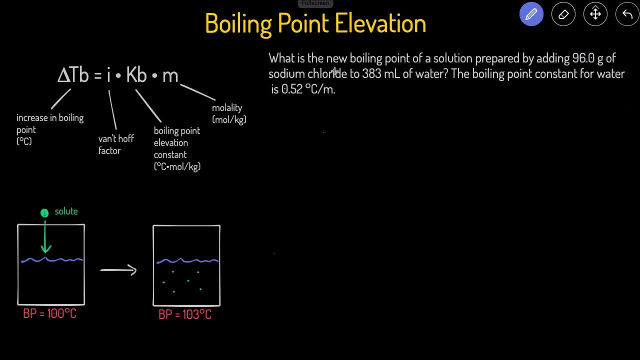 And it tells us the boiling point constant, for water is as such. So our goal is to solve for the new boiling point. To do that, we have to solve for the change in the temperature of the boiling point. So let's start with this equation and take a look at what we have. 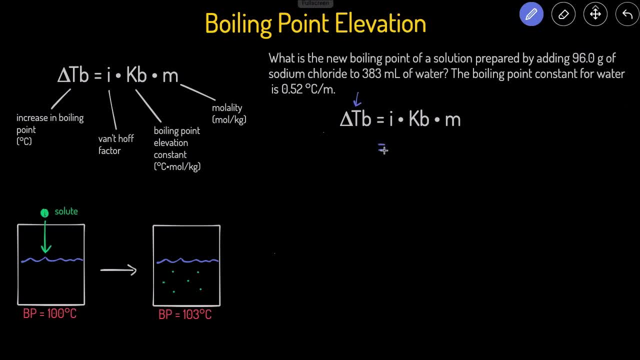 So this is our goal. we're solving for that. I is the Van Gogh factor. it's how many species the solute will break up into. Our solute here is sodium chloride, and sodium chloride's formula is NaCl. This is an ionic compound. 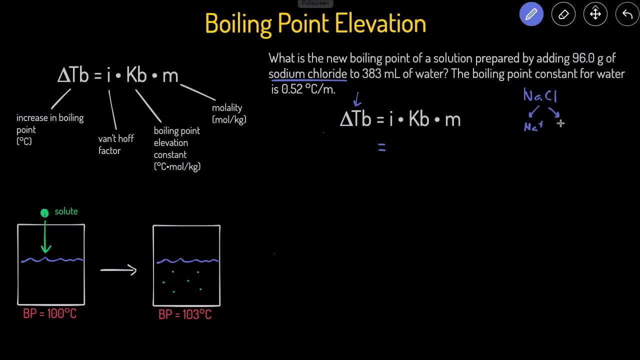 So when this is dissolved in water, it breaks up into Na plus and Cl minus. So you can see, it breaks up into two species. So that means that the Van Gogh factor is going to be two. The Kb- this is the boiling point elevation constant that's given to us as well. 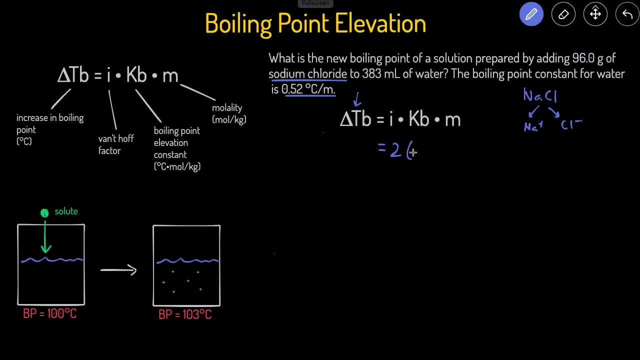 And that's 0.52 degrees Celsius per molal. So I'm going to input that as 0.52 degrees Celsius divided by molal. Then we have to calculate the molality, And molality is equal to 96. And the moles of the solute divided by the kilograms of the solvent. 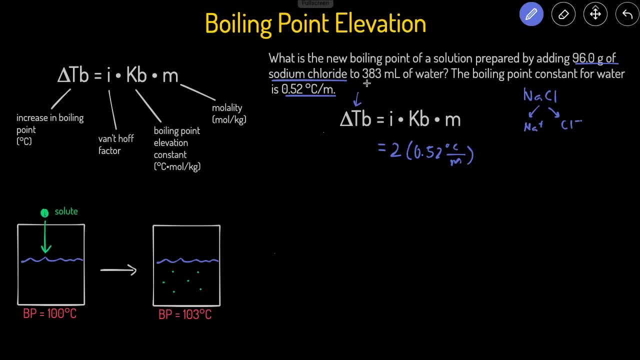 So our solute is the 96 grams of sodium chloride, And then our solvent is the 383 grams of water. Let's start by converting the sodium chloride- the 96 grams of sodium chloride, into moles. So we'll start with the given 96.0 grams of sodium chloride. 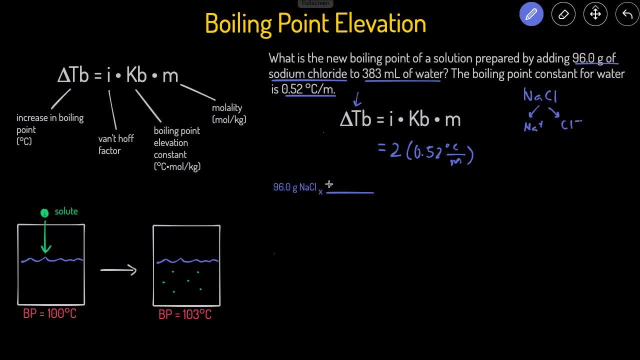 And then to convert it to moles. we're going to multiply it by one mole of sodium chloride over the molar mass. So we can take a look at a periodic table And we'll take a look at the molar mass of sodium chloride. 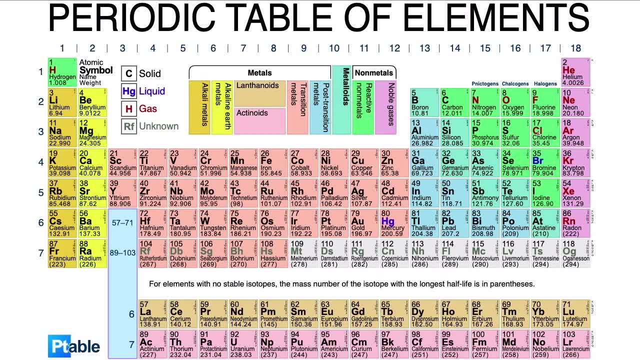 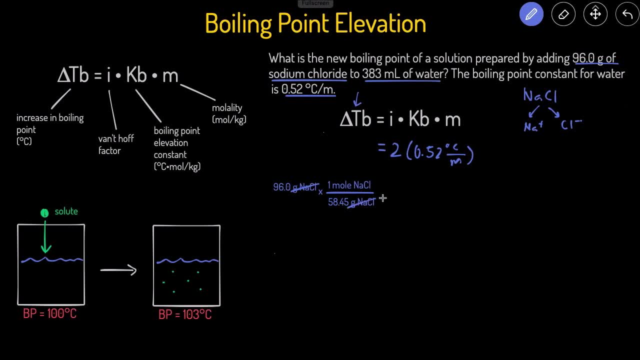 And that just involves adding the molar mass of sodium plus the molar mass of chloride, And that comes out to be roughly around 58.45 grams of NaCl, And then the grams of NaCl will cancel out, giving us moles of sodium chloride. 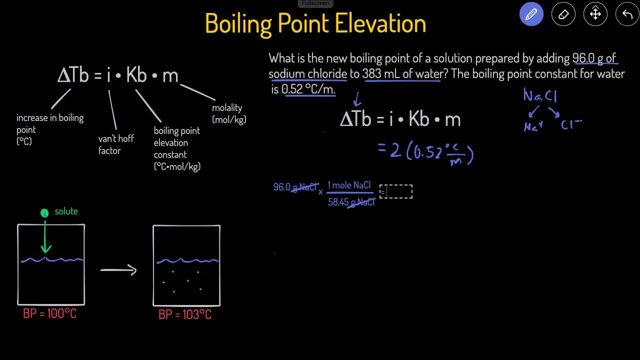 So we'll just do 96 divided by 58.45.. And that gives us 1.64 moles. And then we'll put the NaCl. So now that we have the moles for the molality part, let's figure out the kilograms. 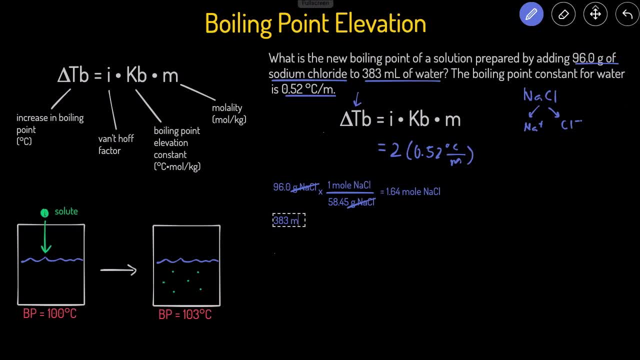 We've got to get the kilograms of solvent, So we have 383 milliliters of water, And then we've got to get this into kilograms. To do that, we first have to convert the milliliters into grams and into kilograms. 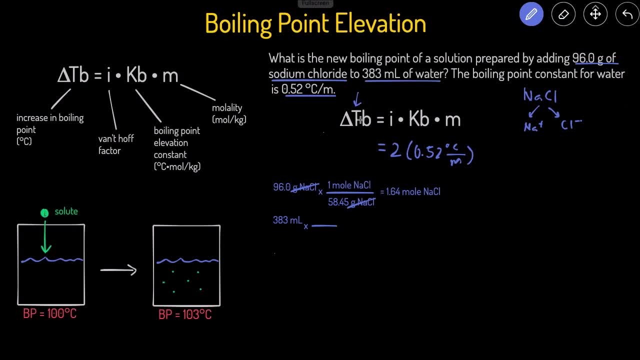 And this is where we use the density. The problem doesn't tell you this, but the density of water is one gram per milliliter, So every one milliliter of water weighs one gram. So we can put one gram on top and one milliliter on the bottom. 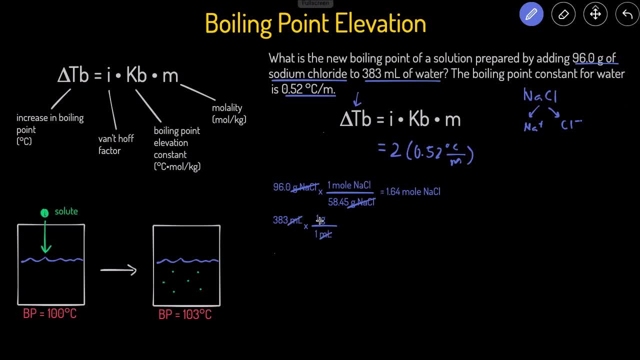 So that means that we have 383 grams of water And then we want to get it into kilograms. For every 1,000 grams there are one kilogram. So essentially, to get the kilograms, we just have to divide by 1,000.. 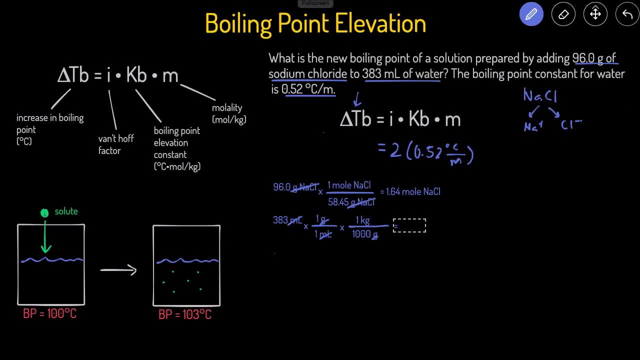 So this is going to be 383 divided by 1,000.. And that gives us 0.383 kilograms. Now that we have the moles and we have the kilograms, we can calculate the molarity. So molality capital M, or lowercase m, is going to equal to the moles: 1.64 moles divided by the kilograms of solvent: 0.383 kilograms. 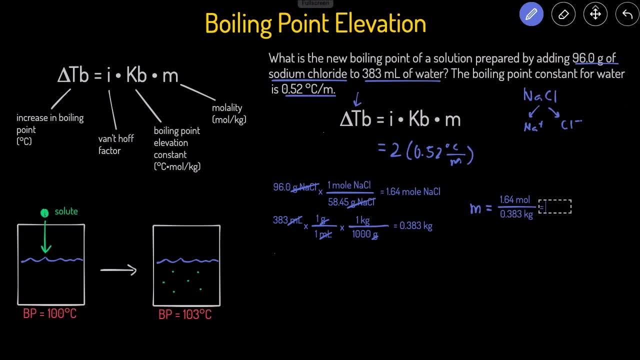 Let's plug that in and see what we get: 1.64 divided by 0.383, and that gives you 4.29 molal, And then that's what you're going to input right here: 4.29 molal for an m. 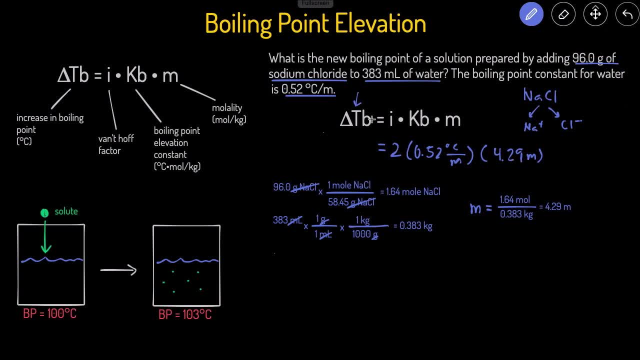 So now we have I, we have KV and we have M, We can multiply these and we can figure out what's the increase in the boiling point, And then that gives you 4.46 degrees Celsius. Or if we're worrying about sick fakes, we should have two sick fakes. 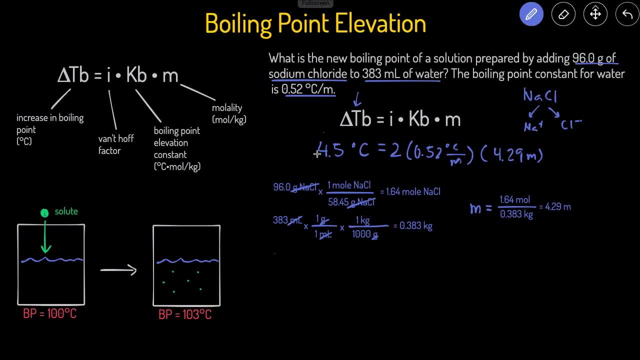 So this should just be 4.5 degrees Celsius. That means that the boiling point has increased by 4.5 degrees Celsius upon dissolving the 96 grams of the solute. So that means our final, our final boiling point is going to equal the original boiling point of water, which is 100 degrees Celsius. 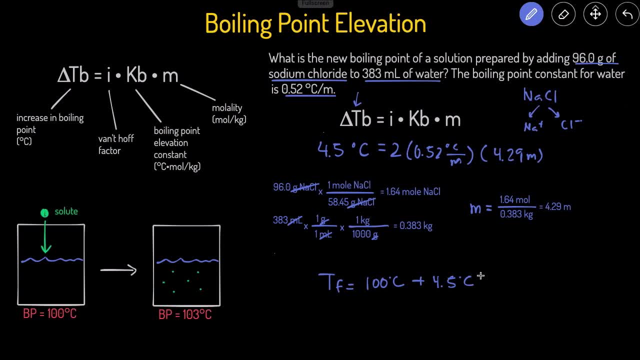 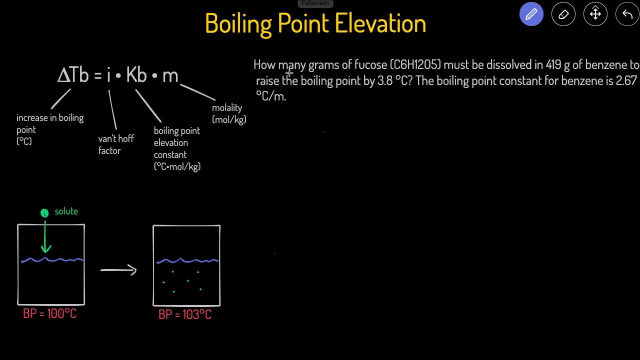 And then we're going to add the change 4.5 degrees Celsius. So that means the new boiling point is going to be 104.5 degrees Celsius. All right, let's take a look at another problem. This next problem is asking us how many grams of fructose must be dissolved in 419.. 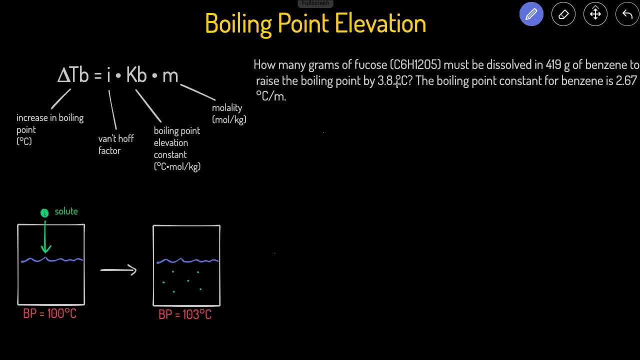 grams of benzene to raise the boiling point by 3.8 degrees Celsius, And then the problem also gives us the boiling point elevation constant for benzene. So, once again, since this problem is asking us about elevating the boiling point, we should use this equation right here. 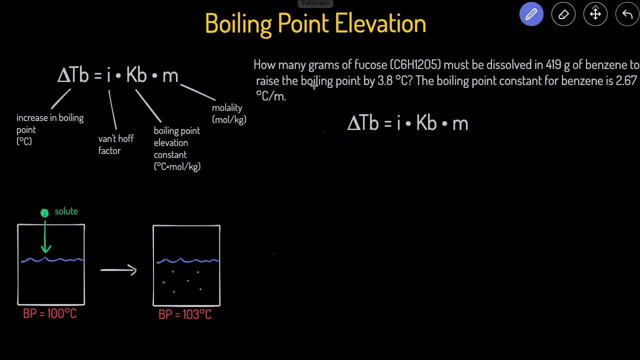 And we already know the change in the temperature of the boiling point. It says that the boiling point was increased by 3.8 degrees Celsius, So we know this is going to be 3.8 degrees Celsius. I against the van't Hoff factor. 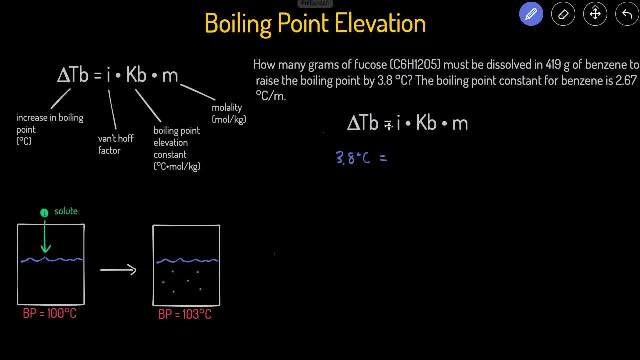 Let's start by identifying which is the solute, What's being dissolved and what's solvent. What's doing the dissolving? We know that fructose is going to be our solute here, because that's what's being dissolved, And then benzene is our solvent. 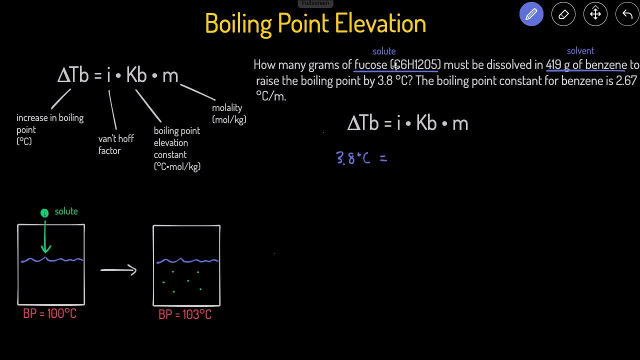 The I value depends on the solute fructose is a molecular compound because it just contains nonmetals only. So we know that since it's molecular, it's not going to break up into multiple species. when it dissolves It stays intact. 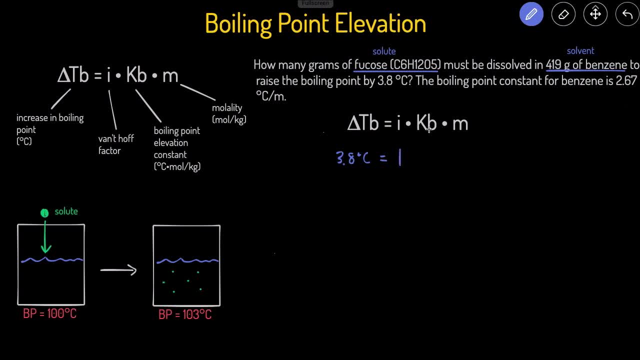 So that means the I value of the fructose is just going to be one Kb. is the boiling point elevation constant? That's 2.67 degrees Celsius per molal. And then the morality. Let's- uh, let's just leave that as our unknown for now, in the sovereign morality. 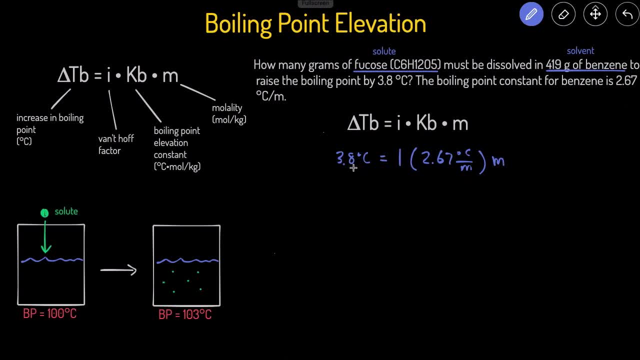 So to do this, we just do 3.8 divided by 2.67, since you were just dividing both sides by 1 times 2.67.. And then that gives us 1.42 molal. Remember, Molal is equal to the moles of the solve, of the solute, which in this case is our fructose C6H12O5, divided by the kilograms of the solvent, which is the benzene. 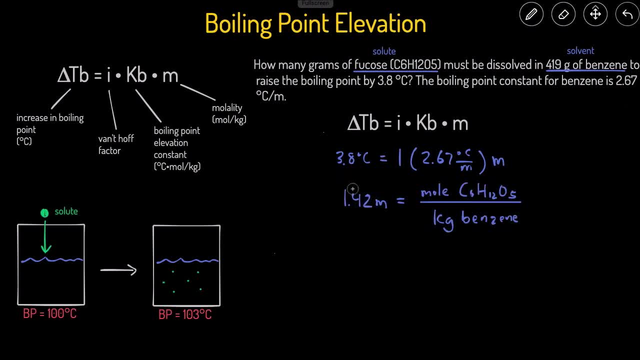 Then let's start substituting some numbers in. I'm just gonna be re copy this down here: We know that the grams of the solvent is 419, so we can divide that by 1,000 to get the kilograms, and that would be 0.419 kilograms. 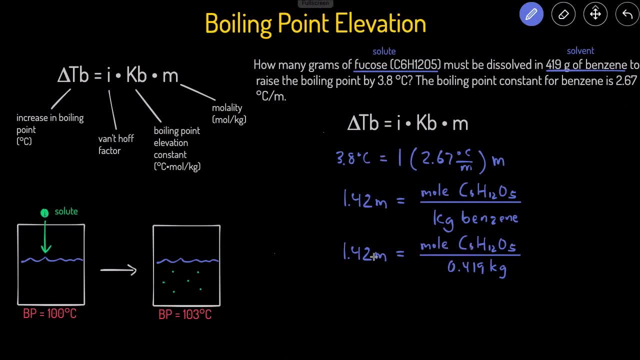 And then we can solve for the moles of the fructose. So do that. We could just cross, multiply both sides, So 1.42 multiplied by 0.419.. And that gives you 0.5.. 595 moles of the fructose. 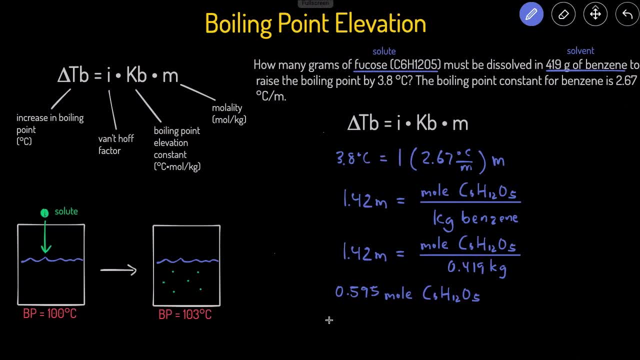 And so, now that we have the moles, to get the grams, we just multiply it by the molar mass, And so we can just calculate the molar mass by adding the six carbons together, the 12 hydrants together and then the five oxygen together.